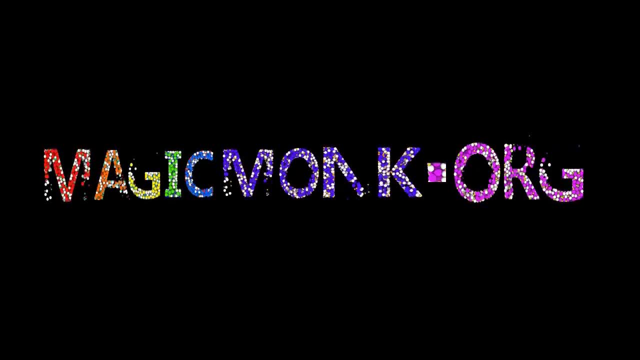 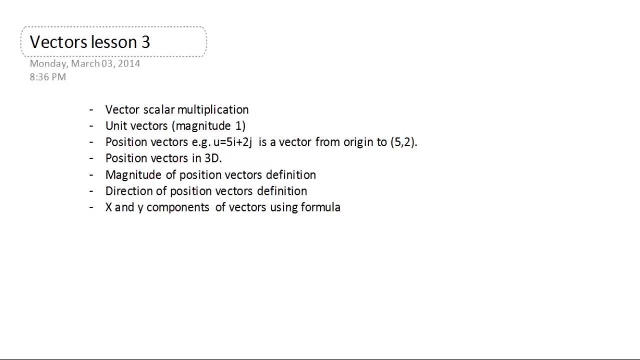 Hey guys, this is Eddie the Magic Monk. Welcome to another vectors lesson. These are the things that we're going to cover in today's lesson, provided that we get enough time to go through them. So let's get started. Okay, so firstly, I'm going to draw a vector And let's call. 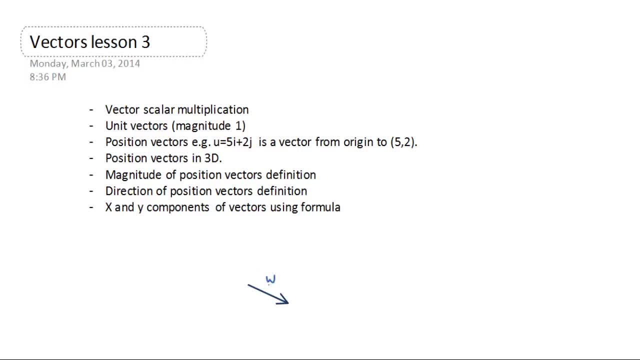 this vector w. Okay, so scalar multiplication means that we are going to keep w in the same direction but we're going to multiply it by a number that increases its magnitude but doesn't affect the direction. So three times vector w would be the same vector. 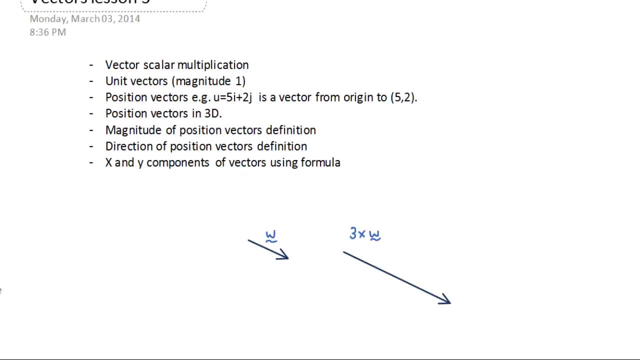 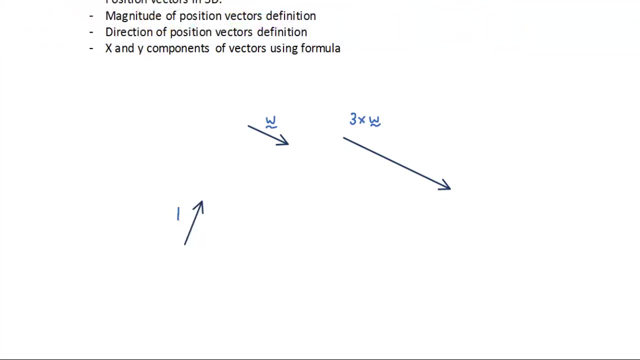 so I'm going to copy it again. But I have increased the magnitude or the distance of the vector by three times. So that's vector scalar multiplication. So let's try to see if you can do one yourself. So I have drawn here vector k And it's going in this direction. 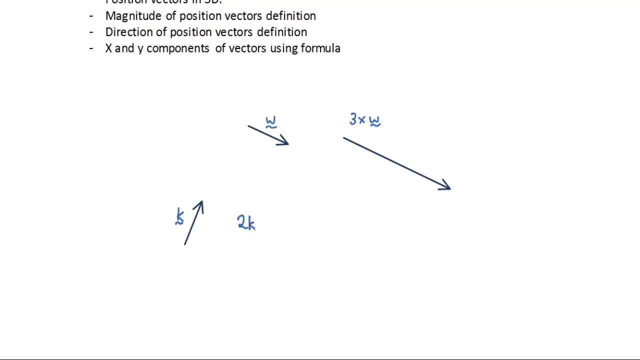 And I want to see if you can do it. Okay, so when I do this, we're going to write vector k, that's vector equal to 2k. Okay, so get that done, come back when you're done. So, therefore, the answer is, if you copy this: 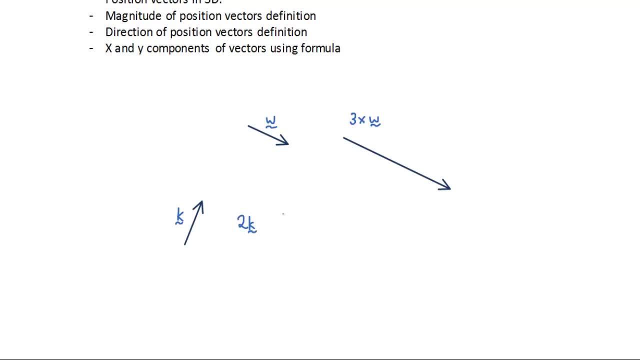 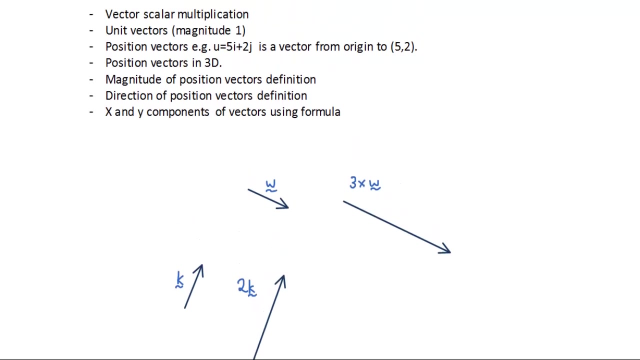 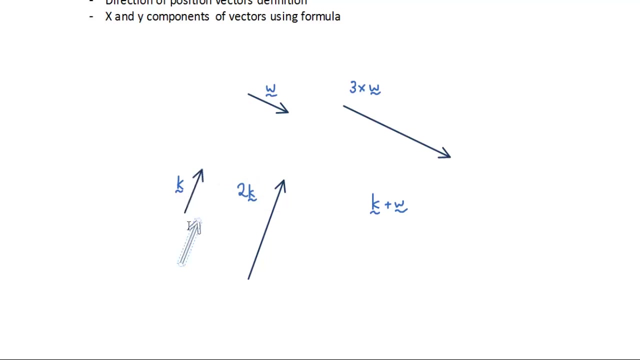 vector again, but extend the length by two, by a factor of two. it should look something like this: Okay, so therefore we can do vector addition with scalar multiplication. so if I wanted to do a vector addition like this, let's do K plus W. okay, then you simply copy the vector K and you copy the. 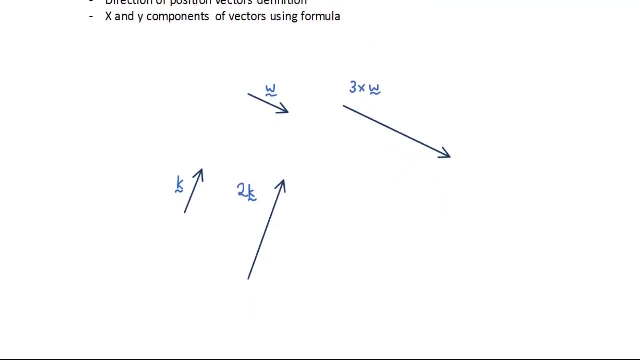 combined with scalar multiplication. so if I wanted to do a vector addition like this, let's do K plus W. okay, then you simply copy the vector K and you copy the vector W, so K plus W, and then you draw a resultant vector from the origin of K to. 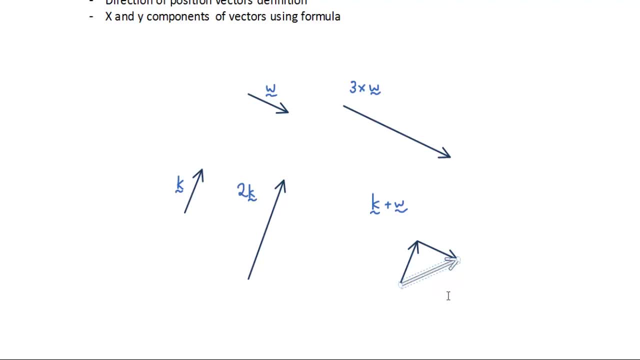 the ending of W, and you can draw a double arrow here if you want, which is what my physics teacher did, and then this is K plus W. okay, if you didn't remember how to do that, so we can do that with scalar multiplication. so I'm going to go to vector 2, K, which is here, and I'm gonna 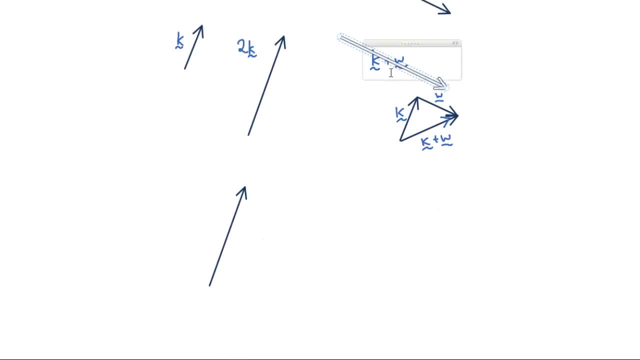 get 3 W, which is that one, so I'm gonna copy it down, and then 2 K plus 3 W, and So 2k, 3w and I'm going to draw a resultant vector between them. so draw a resultant vector. 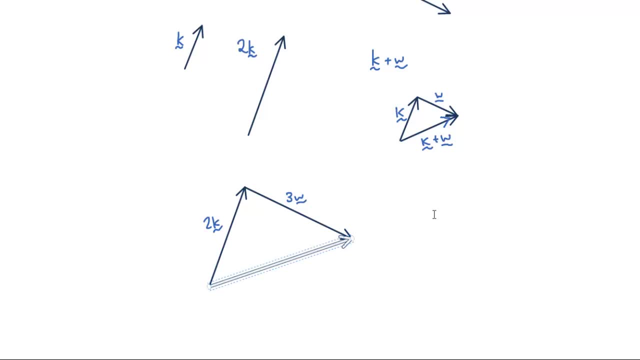 between them, and therefore this is 2k plus 3w. That's what this line represents. Okay, now what if we did 2k minus 3w, So we can have 2k, which is this one, and I'm going to copy it here: 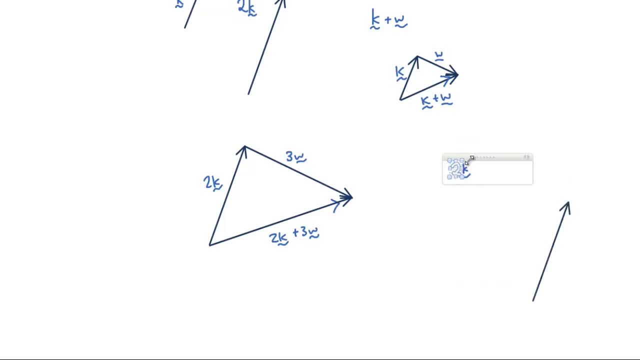 Actually, let's move it down a bit so we have a bit more room. So move this down a bit. And then we have 3w, which is in this direction. so I'm going to copy it again. but if we do minus 3w, what happens is we have to reverse the direction of this vector. 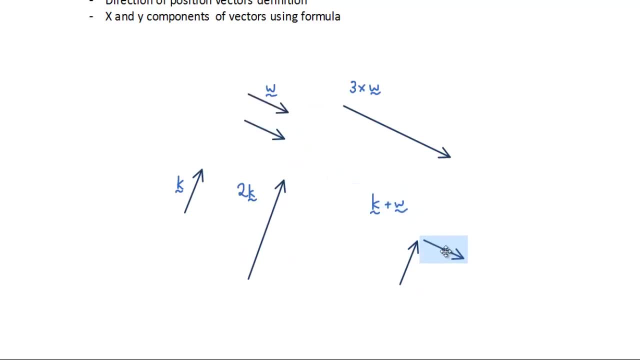 vector W, so K plus W, and then you draw a resultant vector from the origin of K to the ending of W, and you can draw a double arrow here, if you want, which is what my physics teacher did- and then this is the resultant vector, and then you draw a double arrow here, if you want, which is: 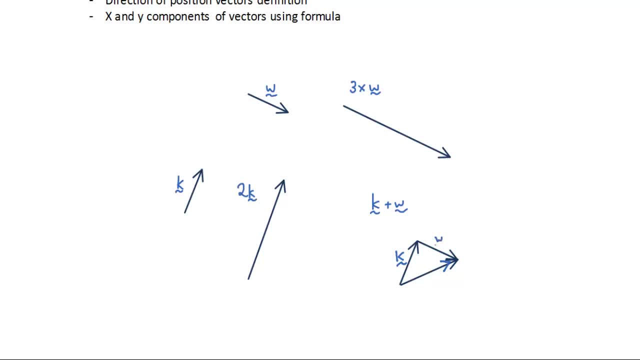 K plus W. okay, if you didn't remember how to do that, so we can do that with scalar multiplication. so I'm going to go to vector 2 K, which is here, and I'm gonna get 3 W, which is that one. so I'm gonna copy it down and then 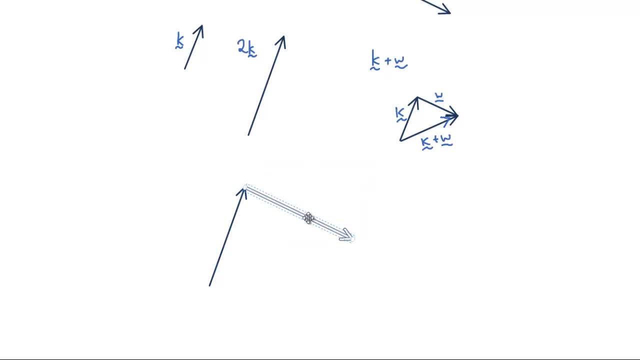 2 K plus 3 W. so 2 K, 3 W and I'm gonna draw a resultant vector between them. so draw resultant vector between them and therefore this is 2 K plus 3 W. that's what this line is represents. okay, now what if we did 2 K minus 3 W, so we can have 2 K, which is: 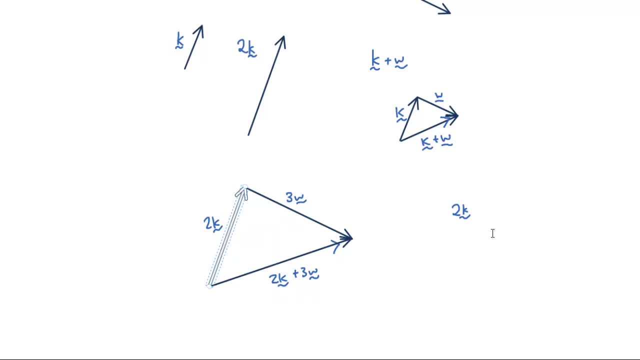 this one and I'm gonna copy it here. actually, let's move it down a bit so we have a bit more room. so move this down a bit. and then we have 3 W, which is in this direction. so I'm gonna copy it again. but if we do minus 3 W, what happens is we have to reverse the direction of this. 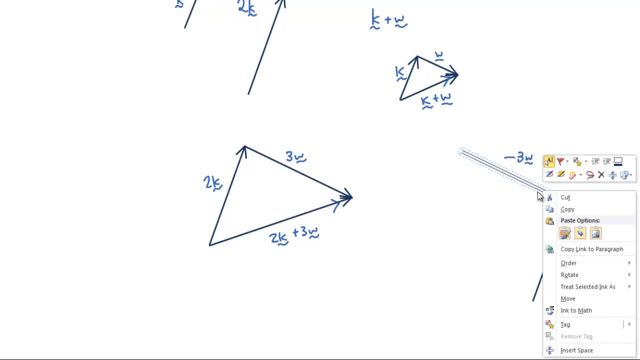 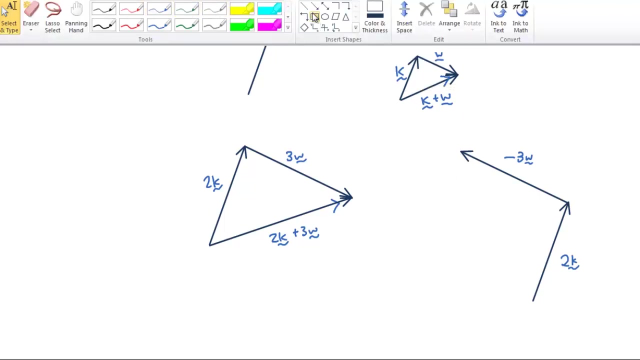 vector. so I'm gonna try and reverse this. so I've just rotated it to the left by 180, so that's reversed it. so I'm gonna just play around here and I think I can do that if I just give it a name, just add one more world or something. so I'm going to add this as my value, and now